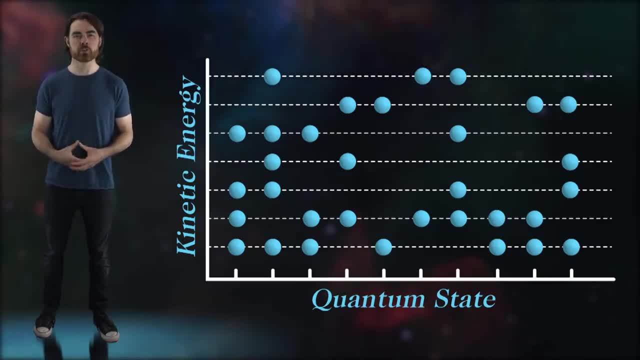 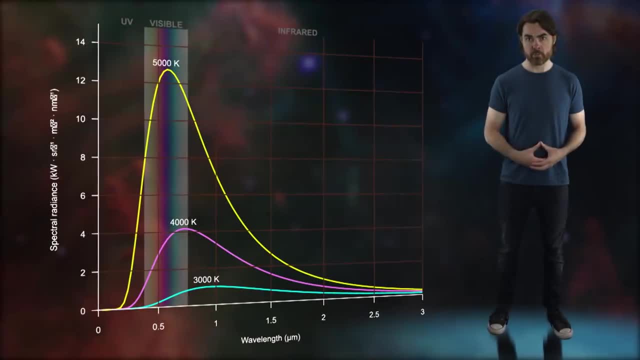 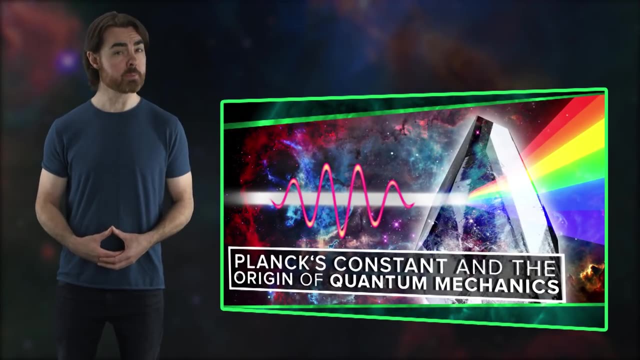 in an atom. This quantum nature is revealed when we look at the spectrum of light produced as those particles hop between energy levels. This is the blackbody radiation described by Planck's law. Its mathematical form was our first hint at the quantum nature of the subatomic world. 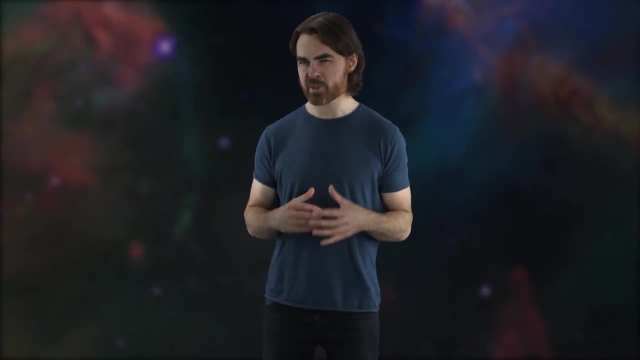 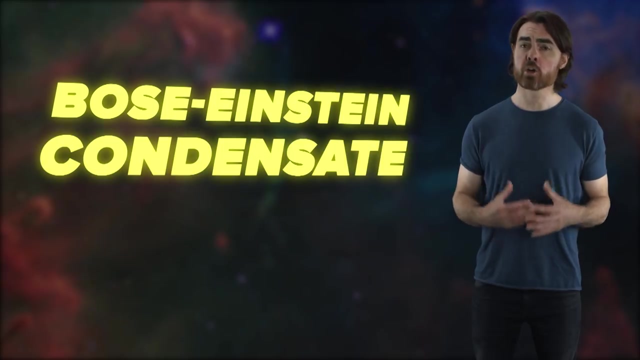 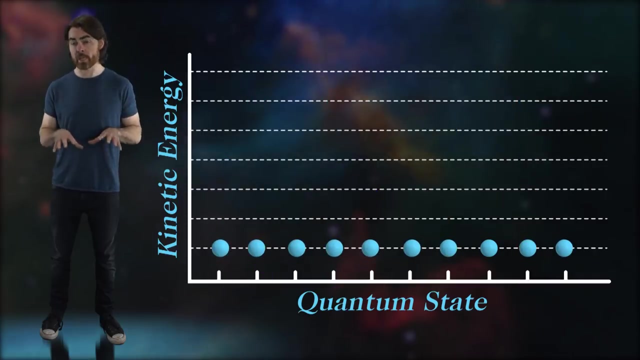 The influence of the quantum world becomes far more apparent in the strange states of matter that exist at the cold end of the heat spectrum. An example is the Bose-Einstein condensate. As we sap energy out of certain substances, its particles drop into the lowest possible energy state. 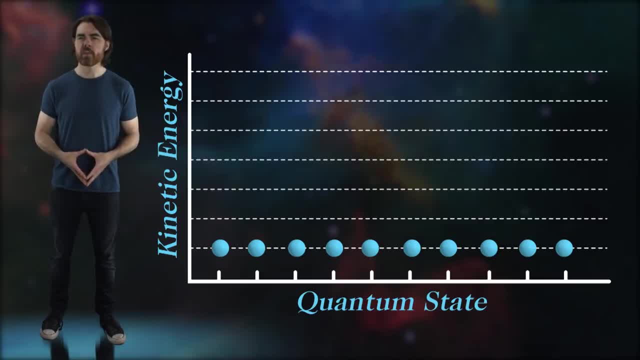 Once nearly all particles occupy that one quantum state, they share a single, coherent wave function. This causes them to behave in a strange collective way. They become immune to individual excitation. Individual particles can no longer be bumped or jostled out of that lowest state. 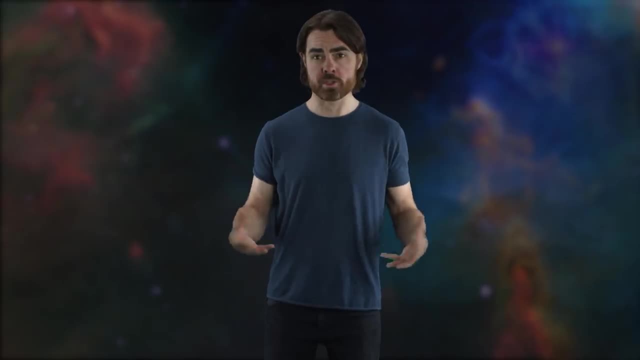 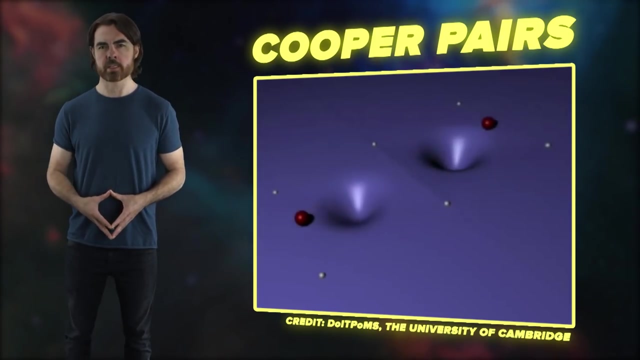 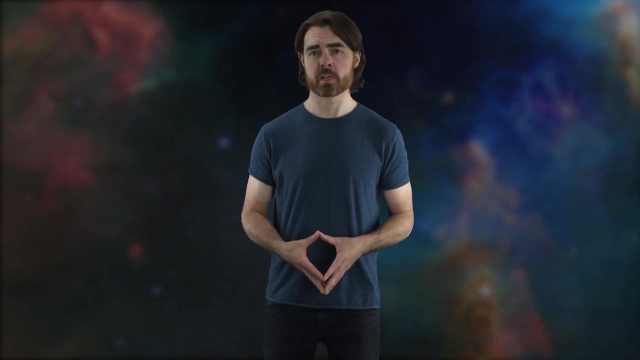 This means that they flow with no resistance whatsoever. In certain solids, bonded pairs of electrons, Cooper pairs- condense into this state. They flow unrestricted through the material, making it a superconductor. However, if the entire substance can somehow remain a fluid when it reaches the critical temperature, 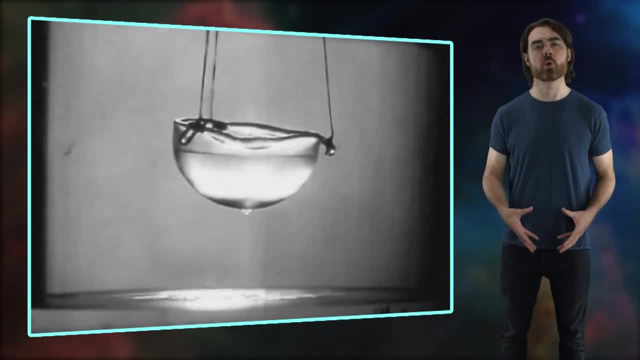 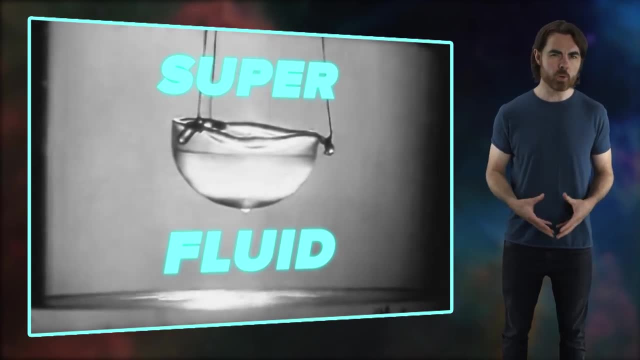 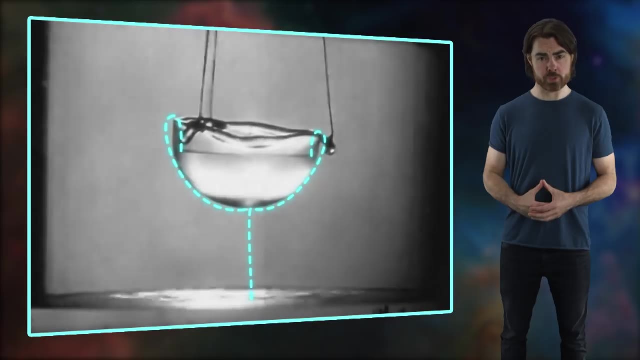 for Bose-Einstein condensation, it becomes what we call a superfluid. It has zero viscosity. It can pass through the smallest openings, sustain whirlpools that last forever and even climb over the walls of its container. Only one substance is known to produce. 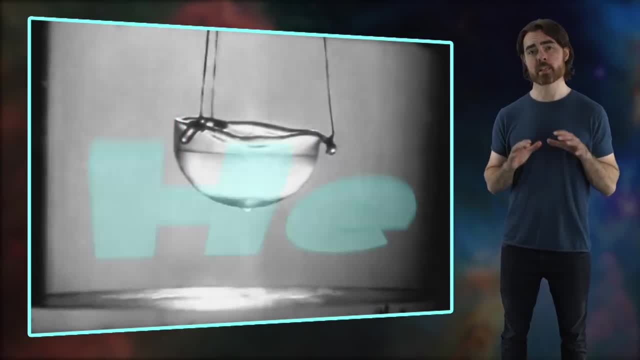 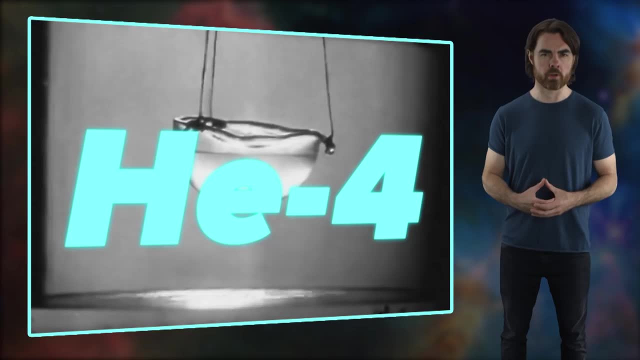 a superfluid for conditions possible in a lab, and that's helium, in particular helium-4.. Helium-4 has a total spin of zero, which makes it a boson, so a particle with integer spin. Now bosons are able to occupy the same quantum state. 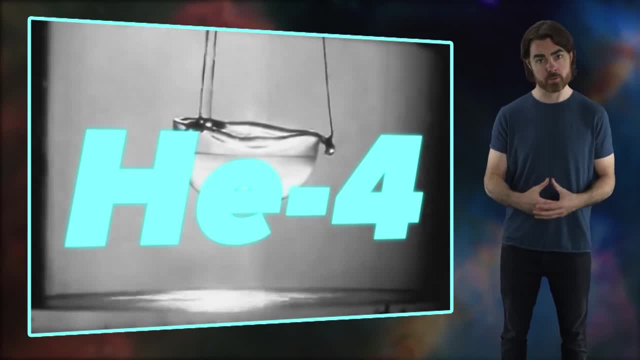 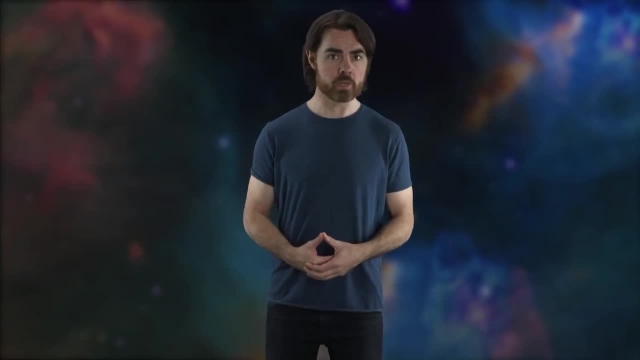 as each other, unlike the half-integer spin fermions, which cannot. The other unique property of helium is that it can't be frozen. It remains a liquid down to the smallest possible temperature. Every other substance freezes into a solid before it can become a superfluid. 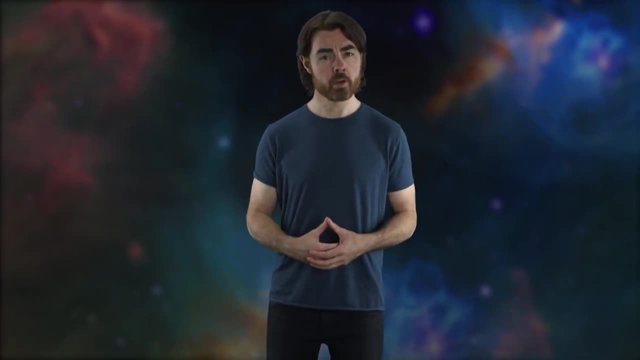 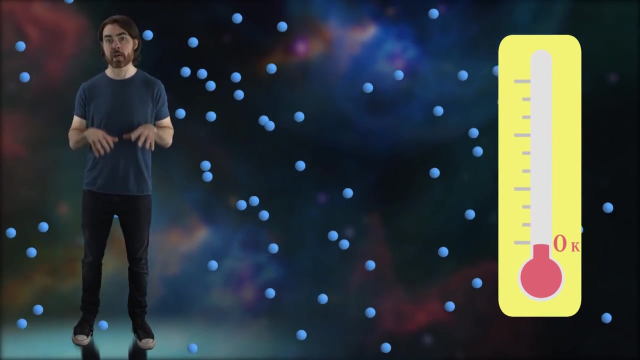 The unfreezability of helium reveals an even deeper quantum mystery. See, there's an absolute limit to how cold a substance can become. In theory, absolute zero temperature means no thermal energy, so no internal motion of particles whatsoever. But what does it mean for a particle to be completely still? 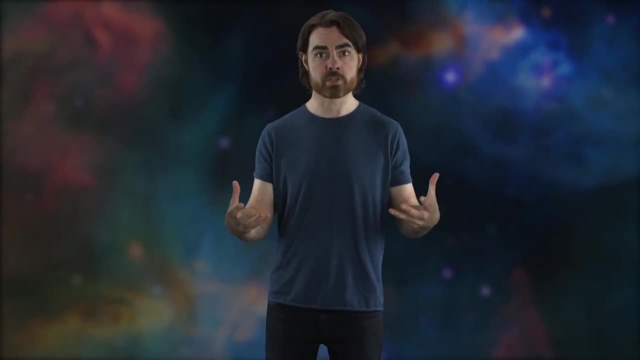 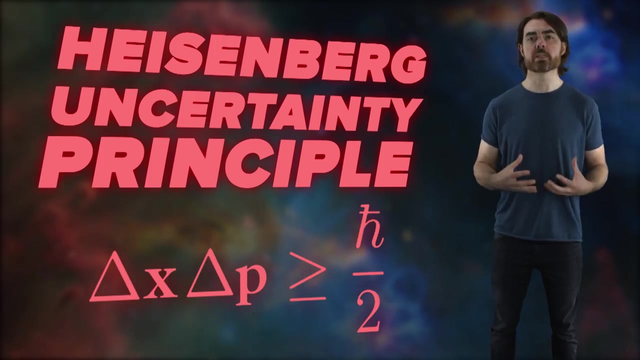 Well, its position relative to its neighbors would be fixed Right And its momentum would be zero. However, the most fundamental law of quantum mechanics forbids this. The Heisenberg uncertainty principle tells us that there's an absolute limit in the knowability of particular combinations of properties. 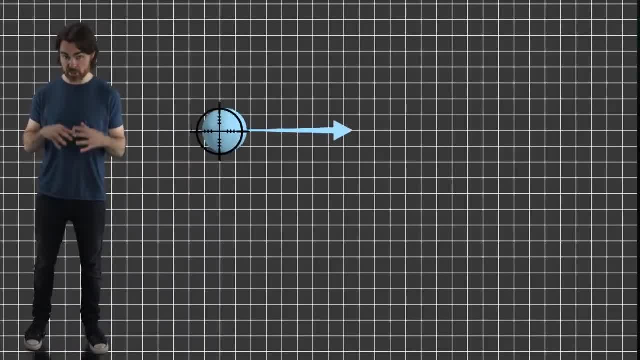 For example, the more precisely a quantum particle's position is defined, the less defined is its momentum, And this isn't about measurement. A particle with a perfectly defined position has a perfectly undefined momentum. So try to fix a particle's position perfectly. 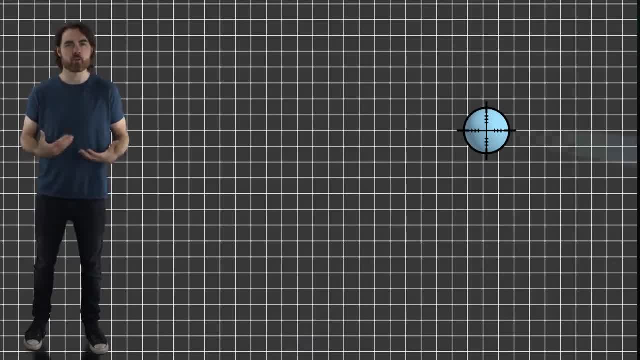 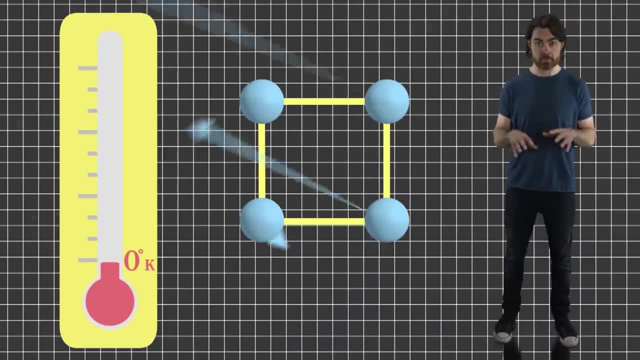 Try to hold it still and its momentum enters a state of quantum haziness. That momentum can then fluctuate, potentially to very high values. At the lowest temperatures. particle motion acquires a sort of quantum buzz. This translates to a very real minimum in average energy. 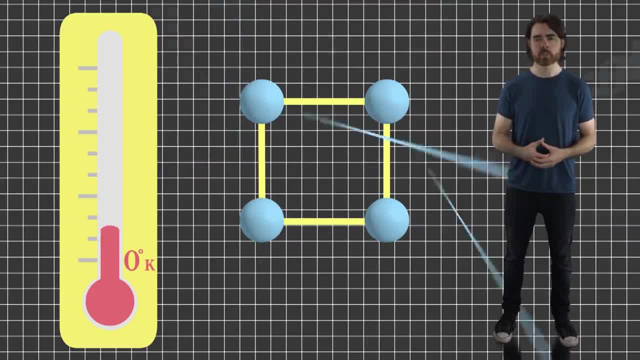 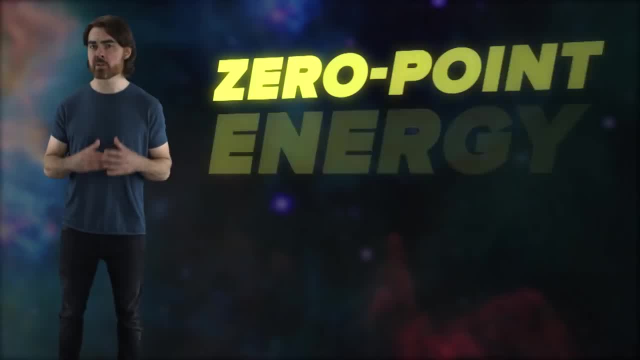 and to a minimum temperature. That temperature is just a teensy bit higher than absolute zero. We call this a quantum buzz. We call the lowest possible energy of a quantum system its zero-point energy For a group of particles that make up any form of matter. 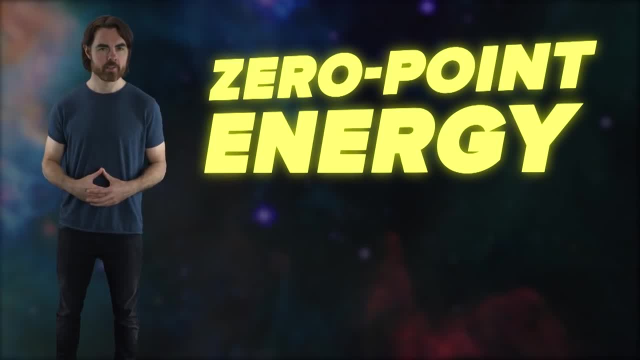 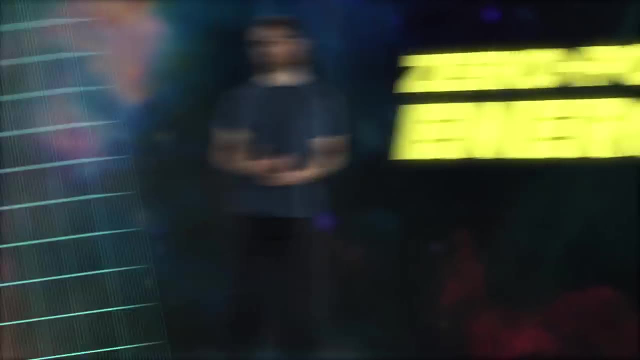 that zero-point energy isn't actually zero. There's always a little bit of kinetic energy remaining, and so it's impossible to reach absolute zero in temperature. Other quantum systems also have non-zero-zero points, and that leads to even stranger phenomena, For example the quantum fields that fill our universe. 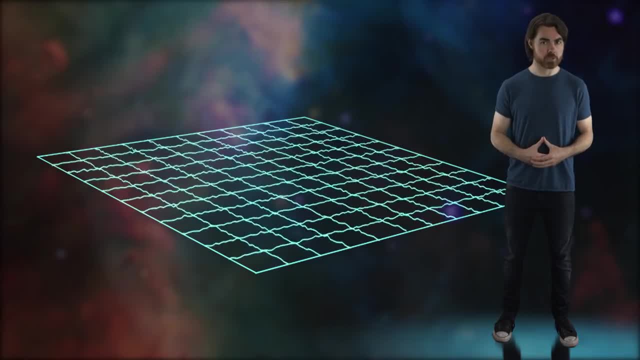 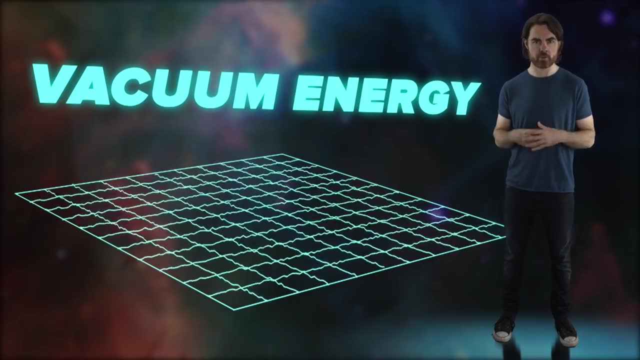 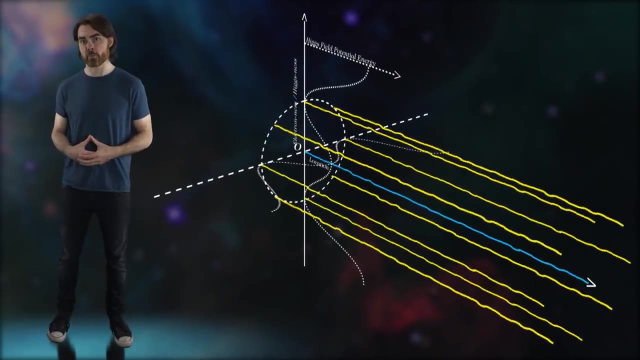 also fluctuate due to the uncertainty principle, resulting in what we know as vacuum energy, And some quantum fields have an intrinsic non-zero-zero point, before even bringing Heisenberg into it. This leads to the famous Higgs mechanism and possibly also the phenomena of inflation and dark energy. 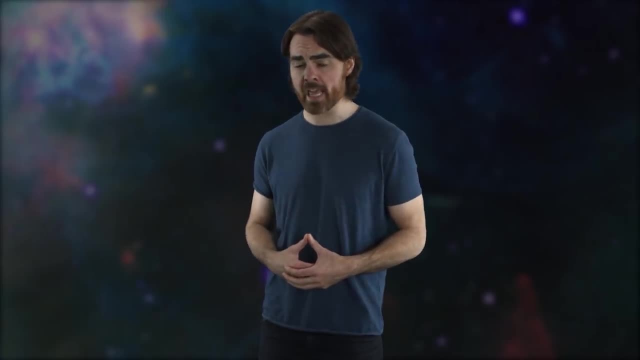 To understand the universe, we need to understand how it behaves absent heat, absent light and absent matter. But we're getting it. We're getting ahead of ourselves. We'll need another episode to explore the quantum nature of nothing, as we peer deeper into the coldest, darkest and emptiest. 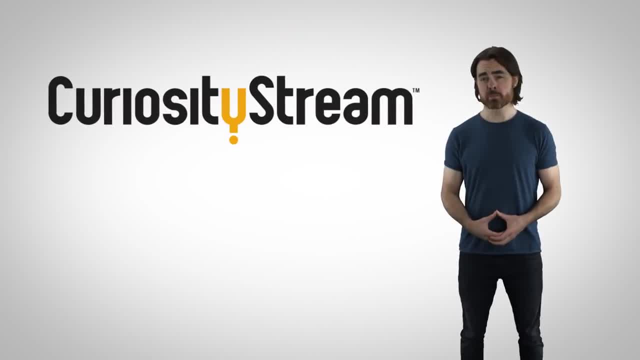 patches of spacetime. This episode is brought to you by CuriosityStream, a subscription streaming service that offers documentaries and non-fiction titles from some of the world's best filmmakers, including exclusive originals. It's also a great place to study up on some of the concepts. 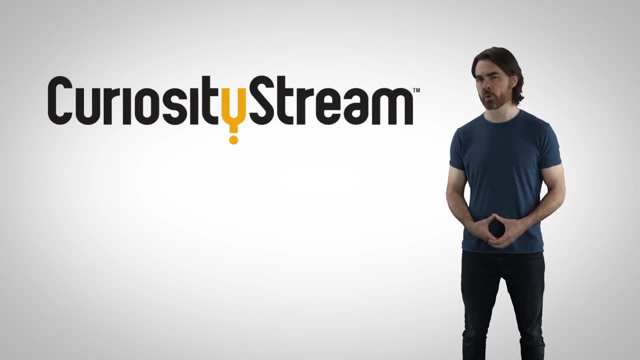 we cover in spacetime. For example, Brian Greene's Exploring Quantum History delves much more deeply into the Heisenberg uncertainty principle. Check it out if you're curious. Get unlimited access today And, for our audience, the first two months. 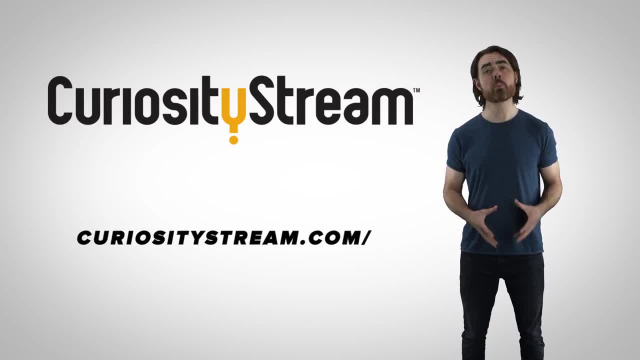 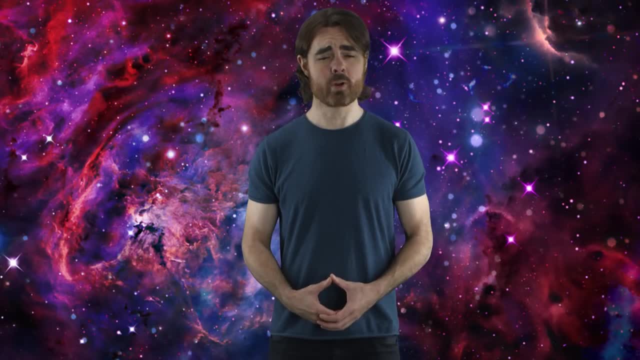 are free if you sign up at curiositystreamcom. slash spacetime And use the promo code spacetime during the sign-up process. This week we hit the crazy milestone of 1 million subscribers. Wow, we never would have guessed we'd reach this point. 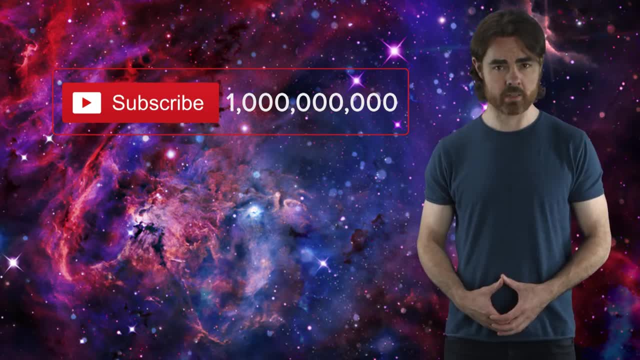 When we started making spacetime early in 2015,, we had no idea there'd be such an amazing community of smart, curious folk out there. We are so incredibly grateful to have found you and that you found us. Of course, we have to give a spacetime t-shirt to our 1. 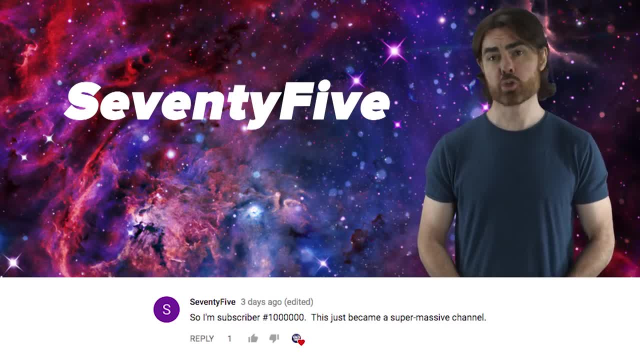 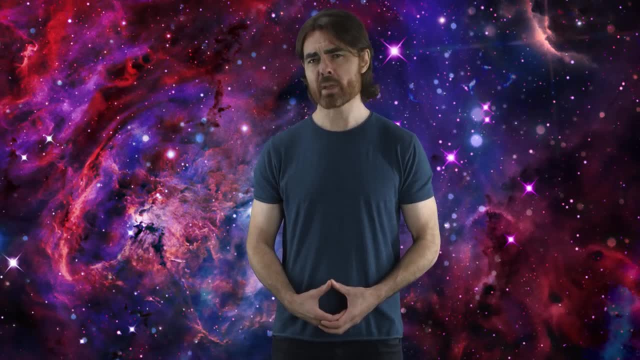 millionth subscriber- 75, that means you Shoot us an email at pbsspacetime at gmailcom and we'll make that happen. And for everyone else, how about we keep making spacetime for as long as humanly possible? 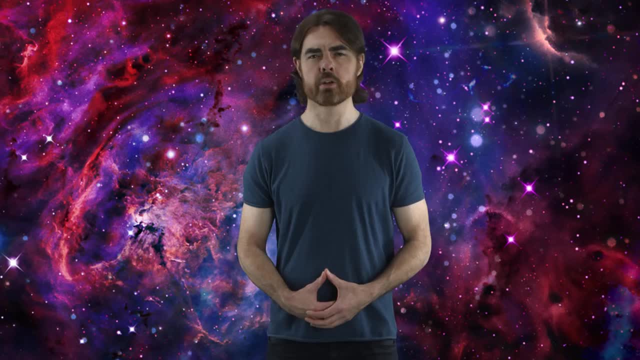 Last week in Spacetime Journal Club we talked about the new observation of a potential pair of binary supermassive black holes orbiting only one light year apart. You guys had the best questions. rcoats89 asked whether we're going to have to wait billions of years for this black hole. 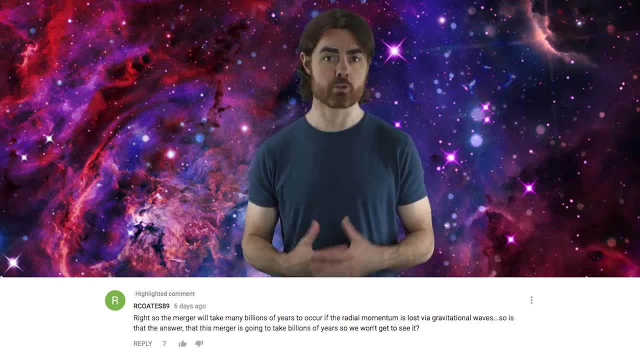 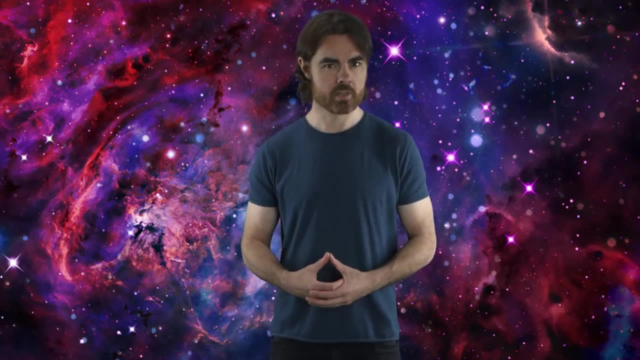 binary to spiral together from losing angular momentum to gravitational waves? Well, the answer is no. We'll probably only have to wait many thousands to millions of years. We know for sure that supermassive black holes do merge, Otherwise they could never have got so big.